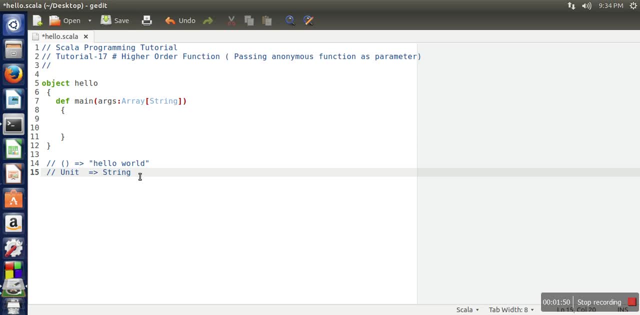 null, like we are not having any parameter. now, let's say you, we are having a anonymous function on this format. so this anonymous function, what it will do, it will return addition of two numbers. so in this case our type of anonymous function will be int. int- put in the braces in the previous case. 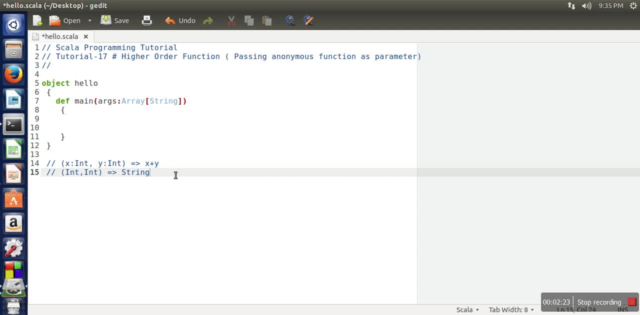 yeah, also, you need to use braces and return data type also. it is int, so this is the data type of this function. so here I am going to write a function, what that function will do. that function will take one anonymous function as a parameter. so let's define that function. I am going to name that function, perform and this: 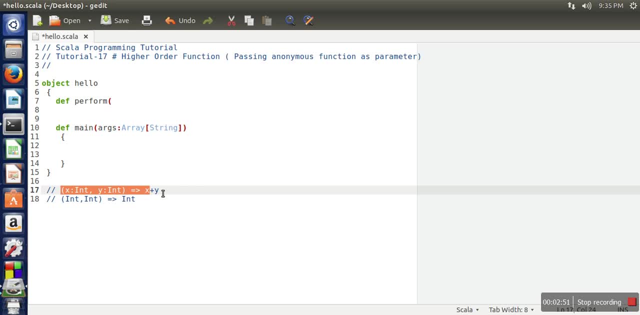 function will going to take anonymous function of this type- sorry, this type. so it will take two parameters and it will return integer value. so in function, let's say this function is having a integer type of parameter, so how will we going to write like f and then int? so first we write the name, that is the place. 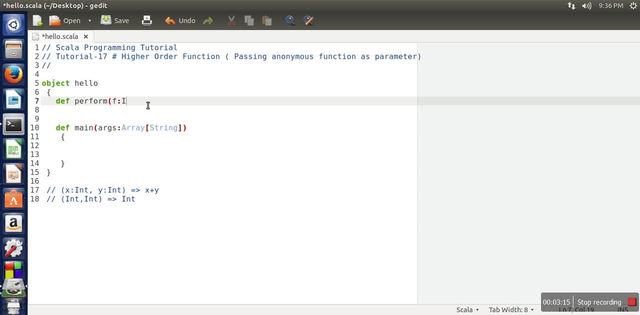 holder, where the value will be stored, and then that data type. so in this case also we are going to do the same thing: name value, because every anonymous function actually you can say, instantiated as a object, so that object will be stored in this F. so here F and 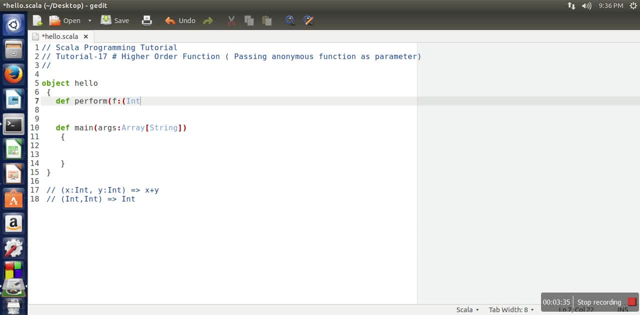 then type of this F. so type will be int, int. and then if you want to pass any parameter, you can pass. but let's say we are not going to pass any parameter and inside this function what we will do, as we can see, this F is having a value of 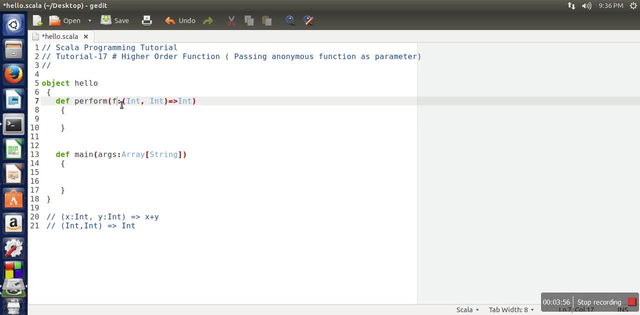 this one. this F is representing the object, and that object can call this anonymous function. so let's call this function on two values, 12 and 23, and here what we will do: we will call this perform function function, and in this perform function we need to pass a anonymous function. what is the type? 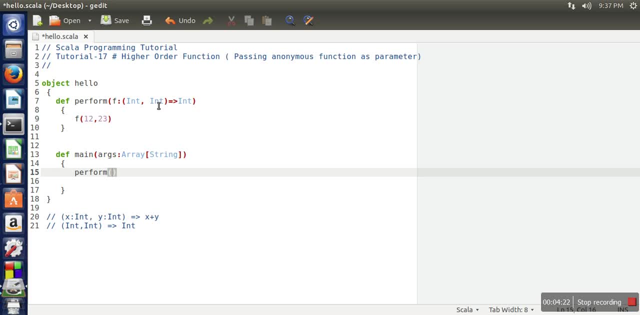 of anonymous function. a anonymous function which take two parameter and return a integer type of value. so here we are going to write our anonymous function and what this function will do. this function will return, let's say, multiplication of those two numbers, and here let's print this value. 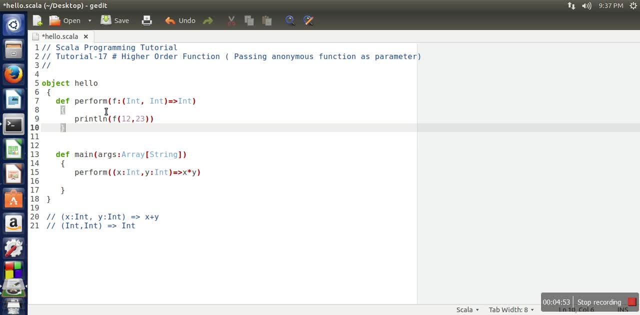 so what we have done, we have defined a function. this function is saying that it needs one parameter of type this one. so this is a anonymous function with two parameter and written type, integer, and inside this one we will call that anonymous function because that function is actually stored in this object. so we, with the help of this object, we will call this: 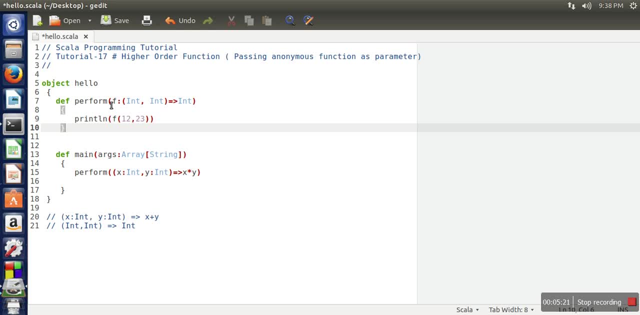 anonymous function and in the main function we are calling this perform and at the place of parameter we are passing a anonymous function. so this function will take two values and it will return the multiplication of those two numbers. so it is fulfilling this type, two parameters, integer- integer data type- and the return type also int. so now let's. 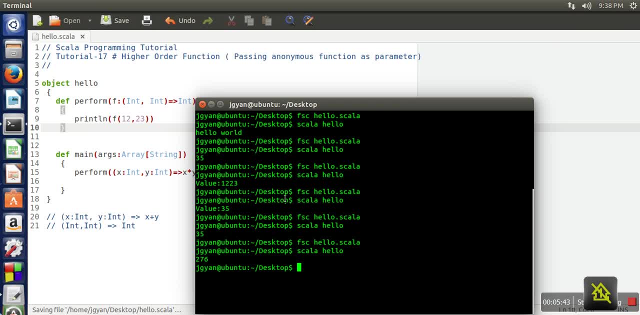 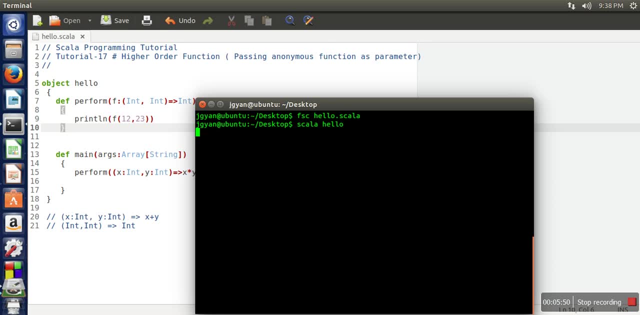 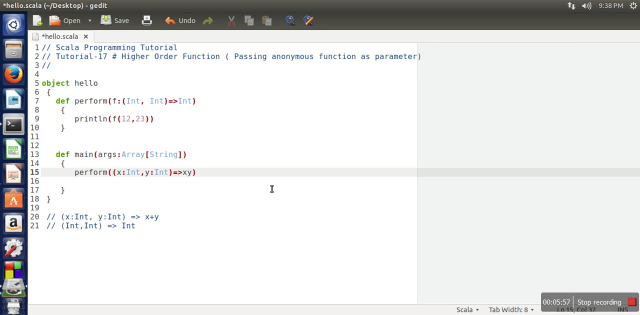 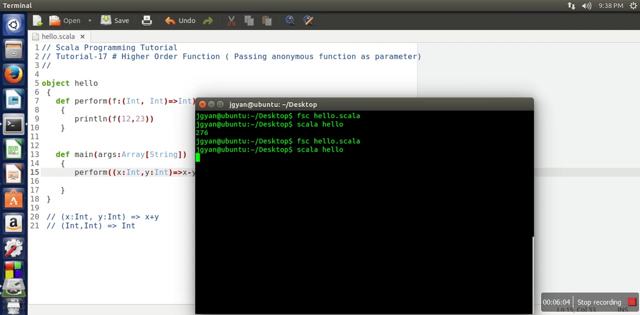 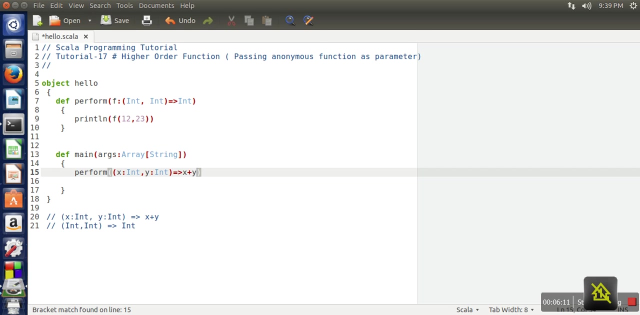 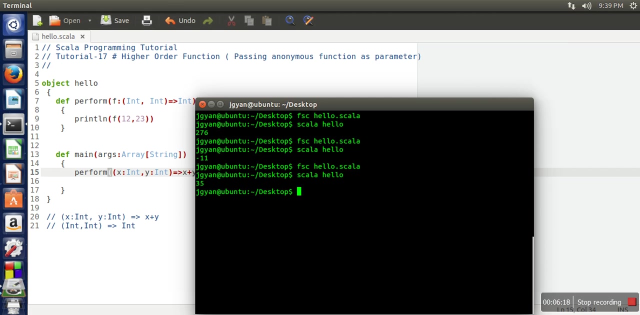 see the output, compile this program and run it. so if you can see it actually returning the multiplication now, let's say, if i'm changing this one to x minus y, so now it's returning the subtraction. if i'm changing this one, compile and then right, so now it's returning the summation. so the thing is that we can change the. 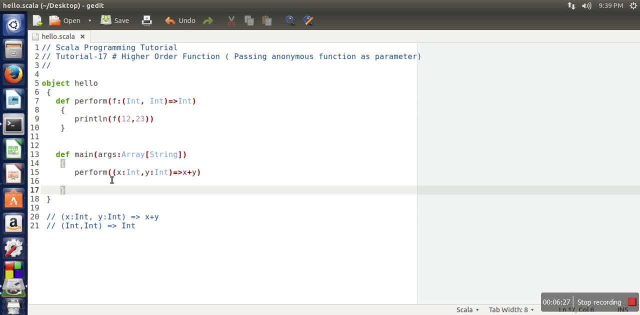 logic at the time of passing argument. whatever logic you want in your function, you can specify that logic here and it will be changed. okay, so this is the simple example of higher order function. thank you very much for watching.